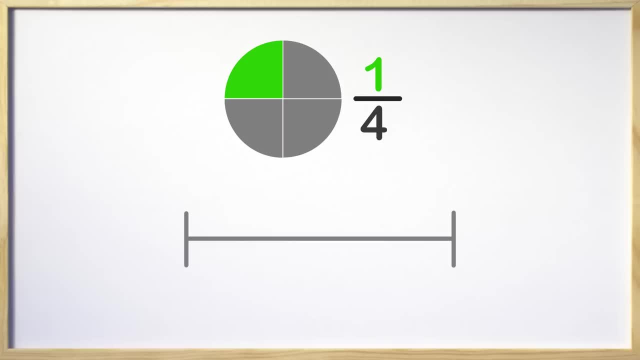 Here is a number line. A number line is pretty easy to draw and you will soon see that they can look a lot like a ruler or a tape measure. Up top we have the fraction we need to represent on the number line. We need to divide the line into the correct number of pieces: The 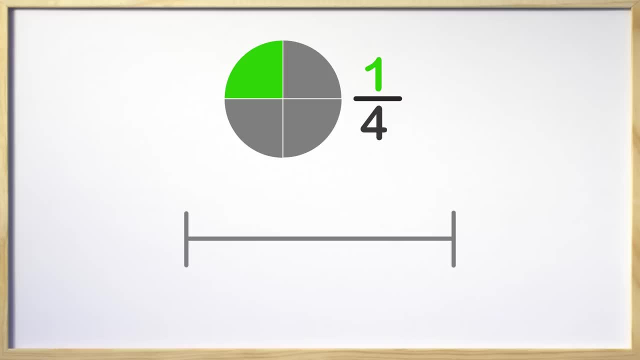 denominator tells us the total amount of pieces. What is the denominator in our fraction? The four is the denominator, so we need to divide this into four pieces. The zero marks the start of the number line. We start at 0.. The number 1 is on the far right. Why do you think? 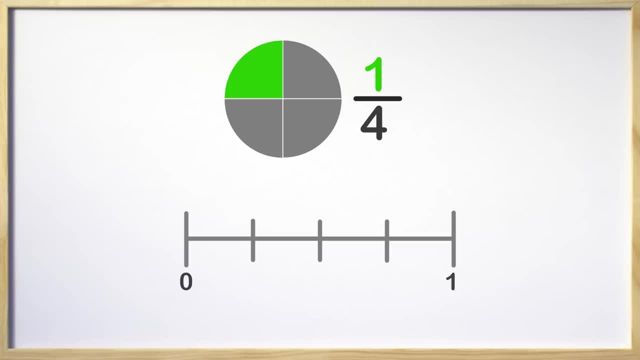 there is a 1 there. The 1 represents the one whole or all four pieces of the fraction above. We could also say that it is 4 fourths, 4 fourths is the same or equal to 1, so that is why we have the 1 here, to show we have reached one whole on the number line This. 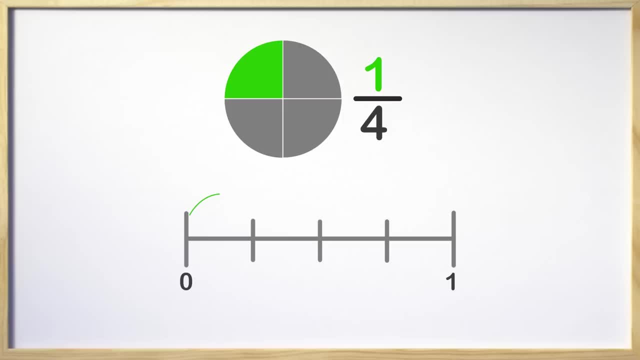 number line is broken into 4 equal parts. From here to here is 1 fourth. From here to here, we have 2 parts, which is 2 fourths. From here to here we have 3 parts, or 3 fourths. From here to here, we have 4 parts or all of them, which is 4 fourths or 1, like we just 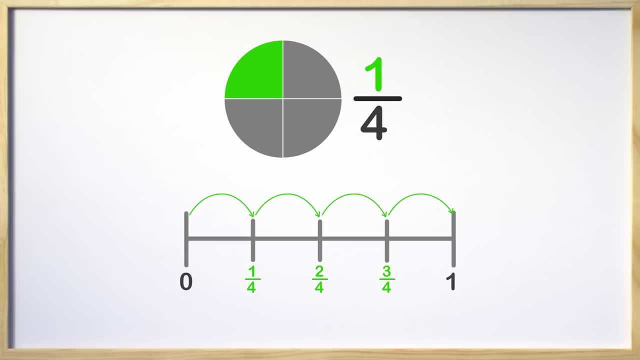 talked about. Something very important we need to remember is when we are counting the fractions on a number line, we are not counting the lines, We are counting the parts in between. The jumps we did with the curved lines shows the parts of the fraction. We now know where 1- fourth is on the number. 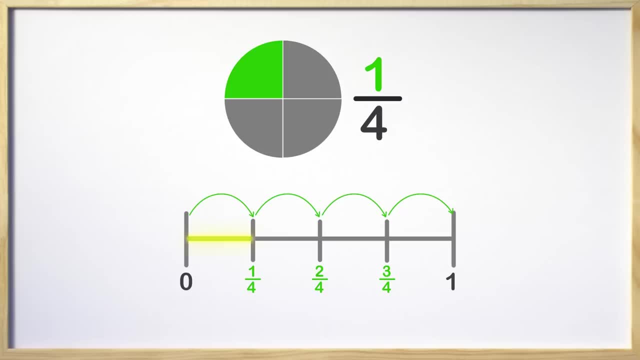 line. It is this part right here. That was great. Let's look at a problem to see if we can solve it. The problem says what fraction is shown on the number line. One way to start this is by finding the denominator in the fraction. Remember, the denominator is the fraction. 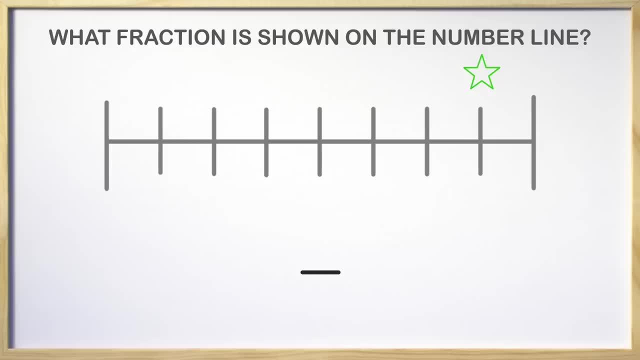 The denominator is the total amount of parts and in order to find that we need to count all the parts, We start at zero and count 1,, 2,, 3,, 4,, 5,, 6,, 7, 8.. We counted 8 parts. 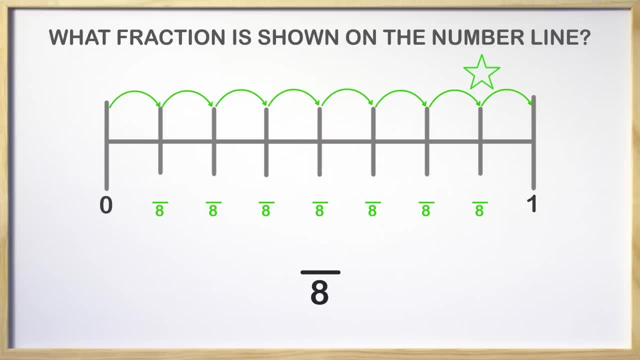 All that is left to do is count the parts up to the green star. Counting again: we count 1,, 2,, 3,, 4,, 5,, 6,, 7, 8.. But we are still counting. Let's try counting again On the second. 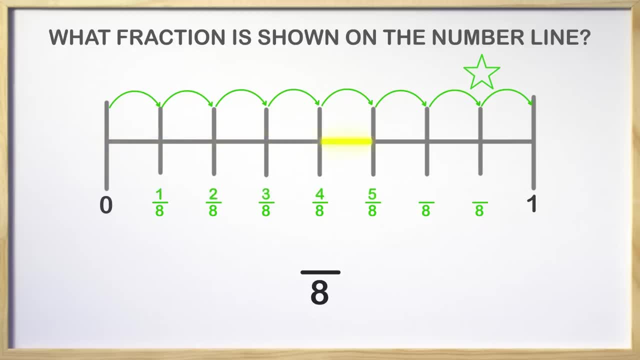 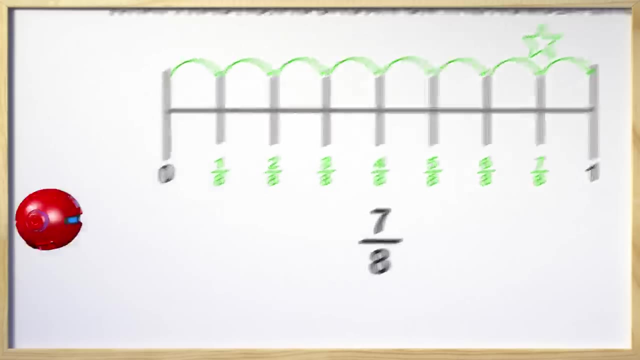 part of the number line. the second part of the number line is the number. with the number, We have both the numerator and the denominator, and the fraction shown is 7 eighths. Great job, guys. Let's take a look at another problem to see how we do. 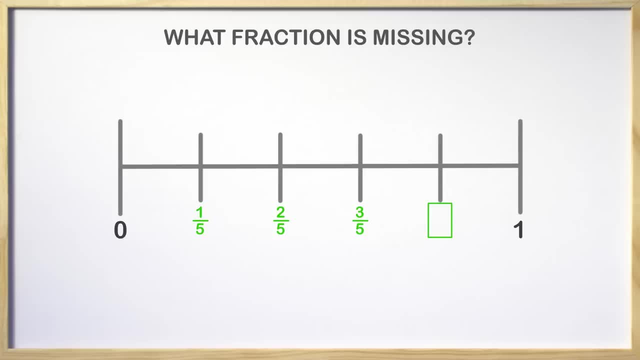 The problem says what fraction is missing In this problem. we know a lot of things already. We know the denominator is 5, so that means there are 5 total parts. You may have figured it out already, but let's count each part on the number line to find. 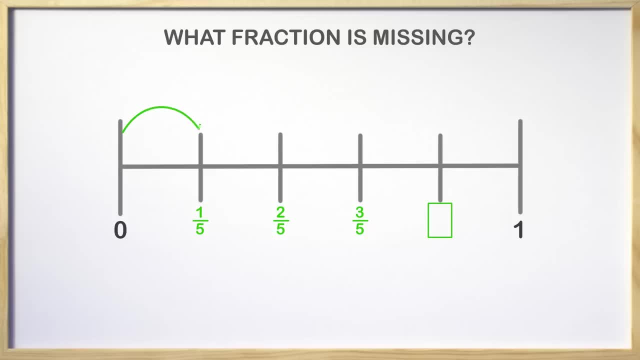 the missing fraction. We count 1 fifth, 2 fifths, 3 fifths, 4 fifths. We have gotten to the missing fraction. What is it? 4 fifths. The missing fraction is 4 fifths. 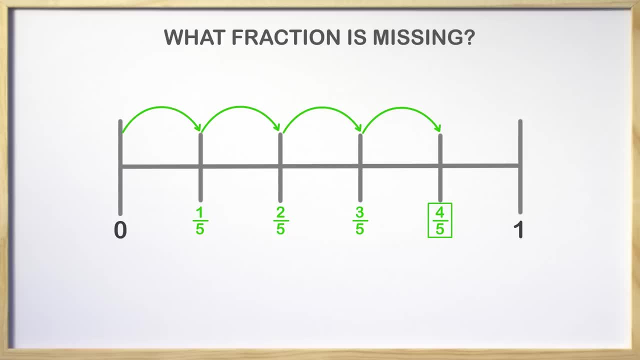 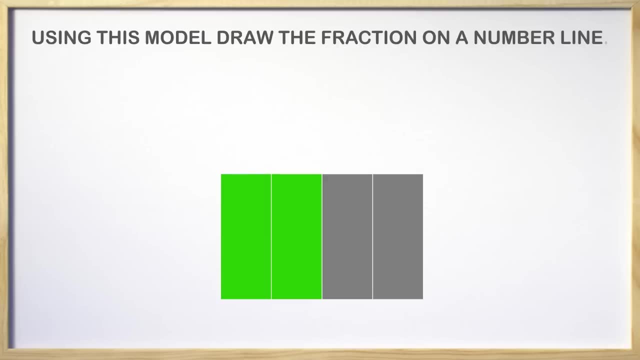 Amazing. We have one last one to do, which will require you to draw your own number line. The problem says: Using this model, draw the fraction on a number line. Take a minute and draw this fraction on a number line, then we will go over it together. 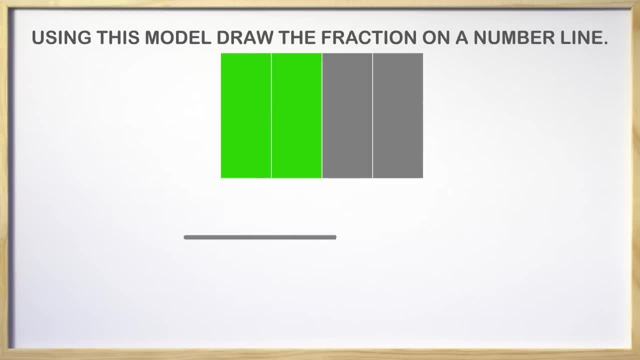 Did you get it? Let's do it together. We have the start to our number line. The zero is where we start and we have 1 at the end, because we are talking about just one whole shape. The denominator is what tells us how many total parts there are. 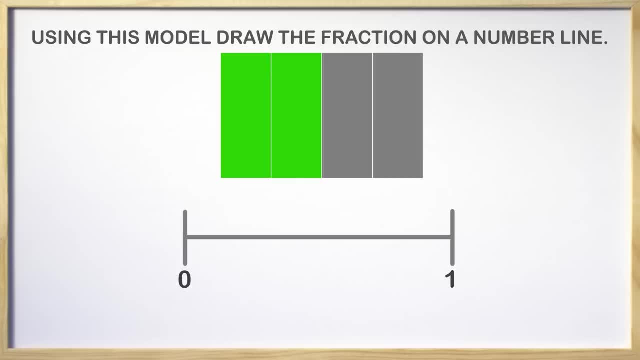 If we count each part of the rectangle, we see there are 4 total parts. so we divide the number line into 4 parts. Looking at the rectangle, two parts are colored green, so that is our numerator. We start counting One, Two. We now have reached the 2 on the number line. 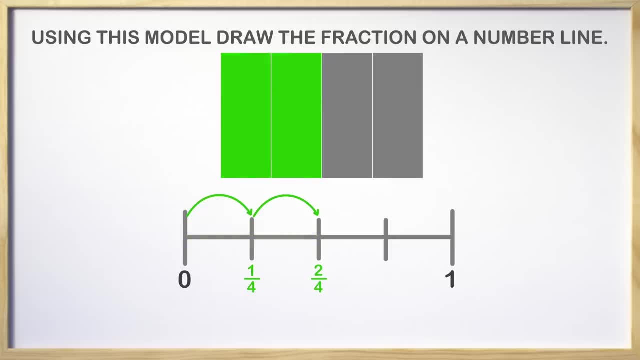 The fraction is 2 fourths. We have shown where 2 fourths is on a number line. Great job. Another cool fact is you can notice that 2 fourths is half way between 0 and 1, which tells us 2 fourths is the same.